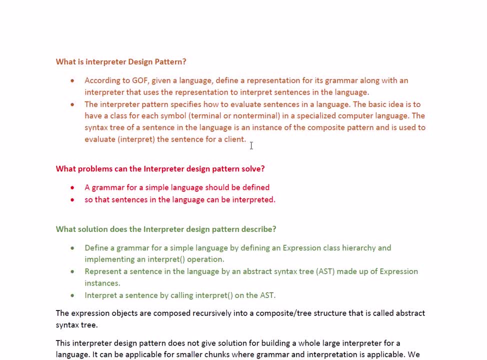 day computer programming languages, basically the way the source code is interpreted, right, If there's an interpreted technology. basically, they also make use of an interpreter in order to understand the source code and translate it into your machine code. Okay, so the basic idea is to have a class for each symbol, terminal or non terminal. Okay, there are two concepts. Terminal symbol means leaves. Basically, if you see a expression, two plus three equal to five. Okay, so this two is basically. 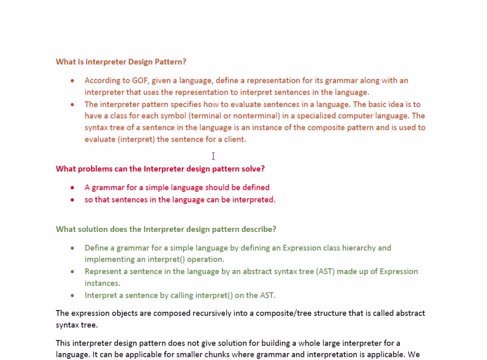 a terminal, Okay. or you can say a leaf node, when it is represented in a syntax tree, Okay. and non terminal or non terminal is one which is basically your operands, Oh sorry, your operators. basically Okay, like plus two, plus three. So in this equation, this plus is basically non terminal, Okay. so these kind of symbols. So terminal is basically most of the time a constant or a variable, whereas non terminal is your operator, Okay. so 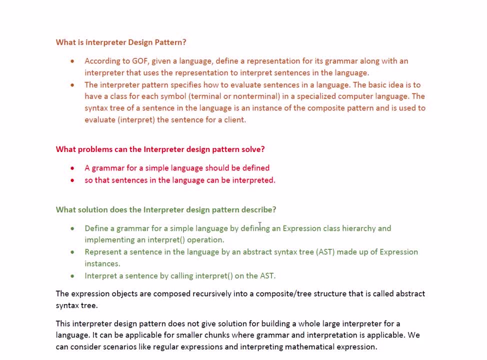 So what problems can the interpreter design pattern solve? So a grammar for a simple language should be defined, Okay. first of all, it aims at providing a grammar for a simple language. Okay, and then, so that the sentences in the languages can be interpreted. Two steps: First of all, you provide a grammar for a language, which we do for all our natural languages, like English, Canada, Hindi, whatever- Okay, so that sentences in the language can be interpreted. 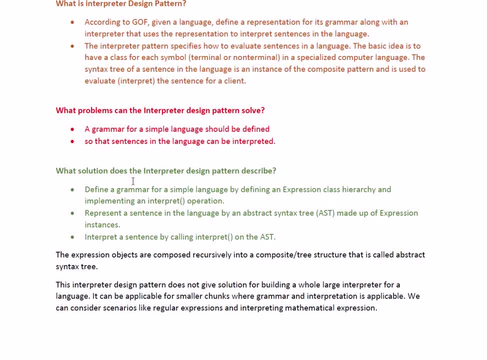 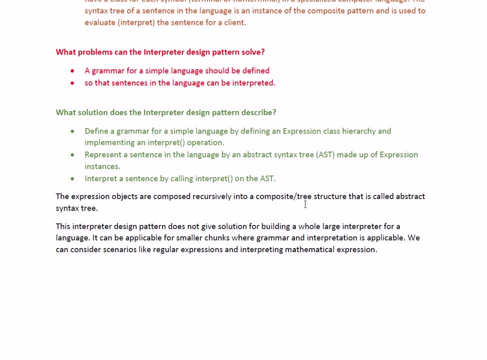 expression objects are composed recursively into a composite or tree structure that is called abstract syntax tree. Okay, this interpreter design pattern does not give solution for building a whole large interpreter for a language. It can be applicable for smaller chunks where grammar and interpretation is applicable. Basically we can consider scenarios like regular expressions and interpreting mathematical expressions. So for this kind of solution- sorry for this kind of problems- basically we can make use of interpreter pattern. 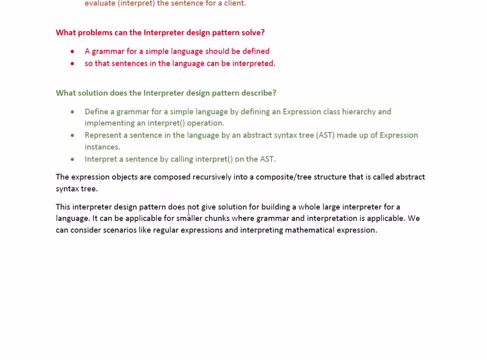 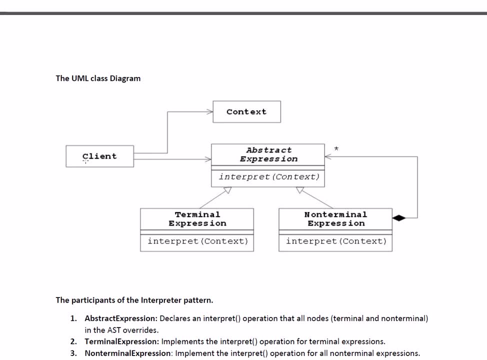 Okay, so let's go through the UML diagram. Okay, so client will trigger. Basically, it's the client application which will trigger this interpreter, So client will be having a context. I'm going to explain this concept soon. The client will contain the context. This context contains the input as well as the expression. Okay, so this context objects is a global object, Okay, you. 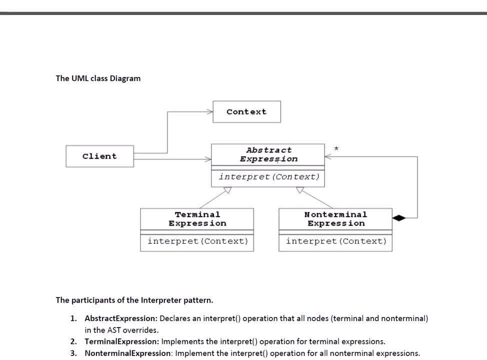 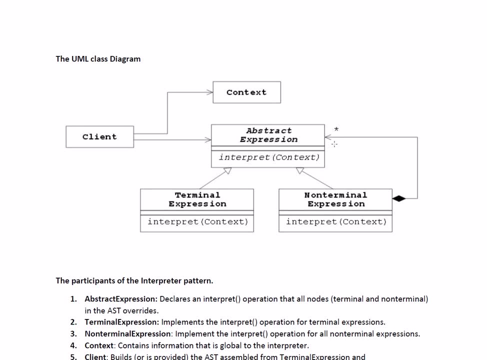 using which basically what we do is we specify various expressions. So we may have in contract or abstract base class, which is called abstract expression, and it contains one method called interpret and you pass a context to that interpret method, Okay, and this global context basically contains the input, Okay, the expression and the desired output, what we want. So, again, an expression can be a terminal expression or a non terminal expression, So two: 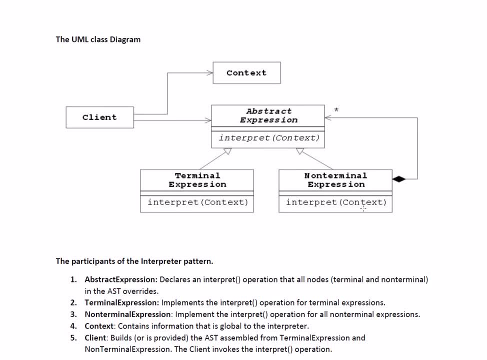 concrete classes basically derive from this. Okay, and again, same operations will be applied on the interpret on the terminal expression. In case of terminal expression, interpret straightaway returns the variables value. In case of non terminal expression, the interpret basically internally calls the interpret method on each expression, You I would say the leave expression or leave expression, and then performs the operator or performs the operation based on the operator and then 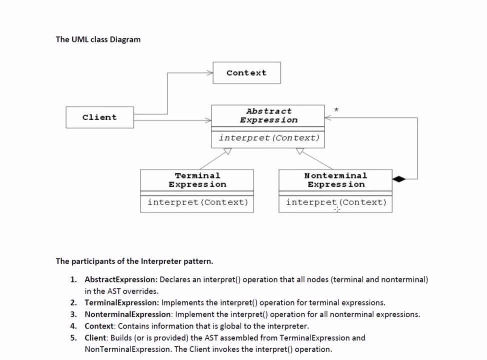 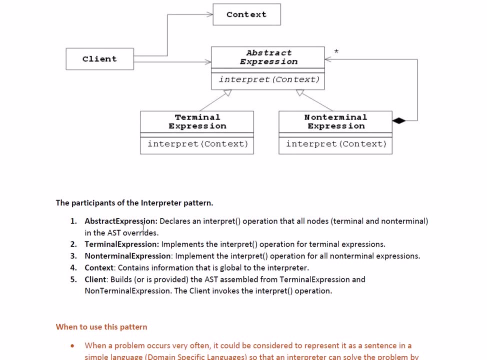 returns the results. Okay, so that's the UML classification diagram for this. So the participants of the interpreter pattern: abstract expression declares an interpret operation that all nodes in the ASD overrides. yes, both for terminal and non terminal. As I already explained, terminal expressions implements the interpret operation for terminal expressions which straight away return of value. non terminal expression implement the intermittent operation in such a way that for all non 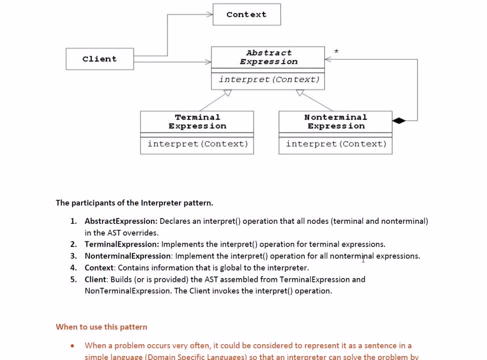 terminal expression. So it basically internally calls this interpret method on each and every leaf node of your non-terminal expression and then applies the operation and returns the result. Context contains the information that is global to the interpreter and the client builds the AST assembled from the terminal expression and non-terminal expression. 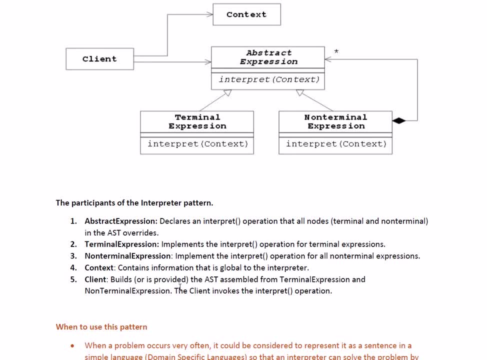 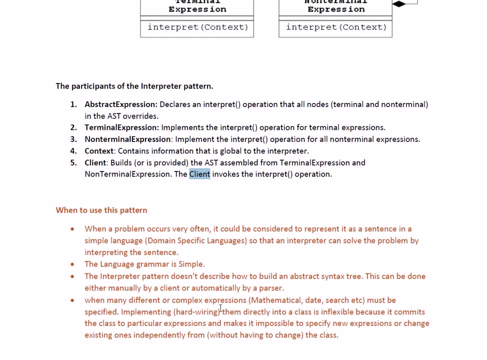 Okay, Basically, it's client who builds or is provided the AST or the abstract syntax tree assembled from a terminal expression and non-terminal expression. The client invokes the interpret operation. This is the entry point most of the time, guys. Okay. So, all that said, let's go through a quick demo. 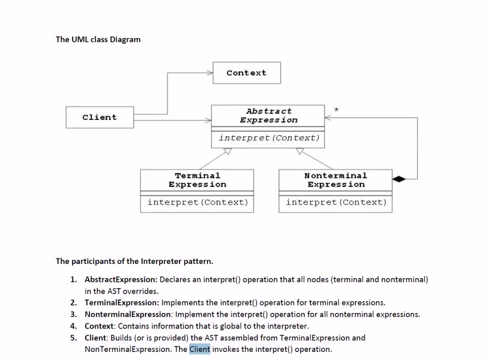 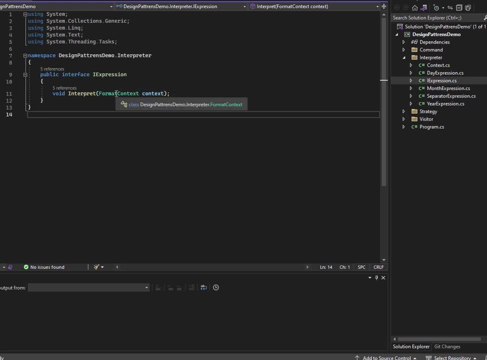 So let's start with the demo. So I'm going to show you. So first thing is I should have a contract or interface called abstract expression. So I have an I expression, Okay So. So it contains one method which called interpret, and I pause. 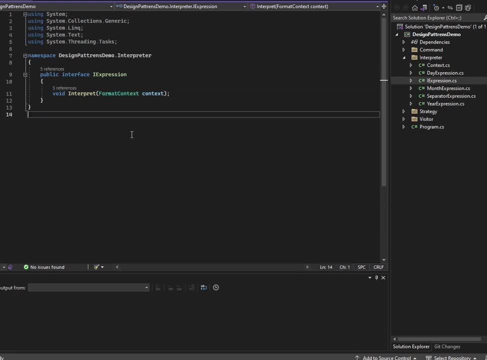 I pass the format context. So basically I have created an interpreter which basically formats the given input value or the given date time string value into the desired format of date time string value which is required for the display. A trivial example: basically, Okay. 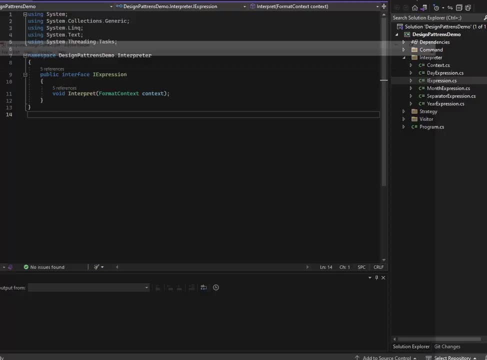 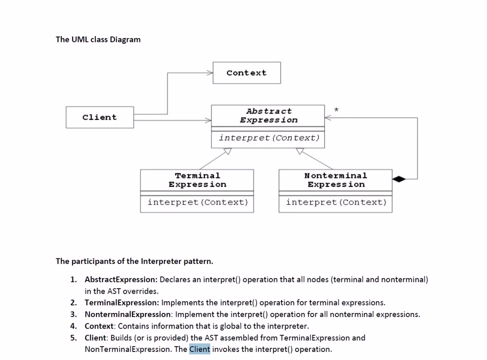 That's why I have a format context. So let's go through the UML diagram. Okay, So this is my abstract expression, which contains one method- interpret- and expects a context, Which I'm passing over here, and then the context, most important thing. 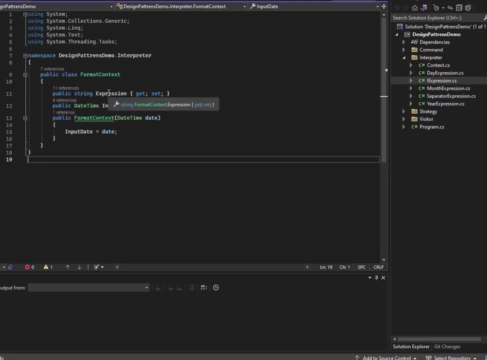 So format context: it contains the expression: Okay, Basically the end result once it is interpreted by an interpreter: Okay, So this is the expression result, I would say. and then date time, input date: Okay, The date I'm passing in order to get the desired output, and then I'm passing for the context. object: 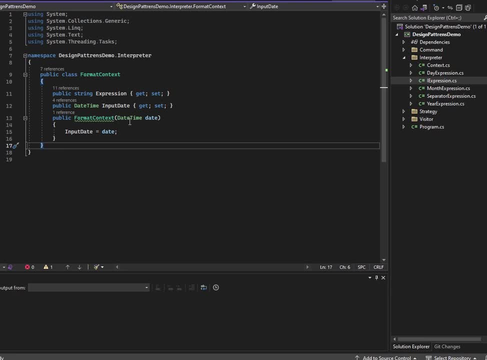 I'm passing the date. basically, in order to get the, The desired date value needs to be formatted Okay. So very simple: context object. And then this is my I expression, Okay, My expression contract. And then let's go through the concrete implementation. 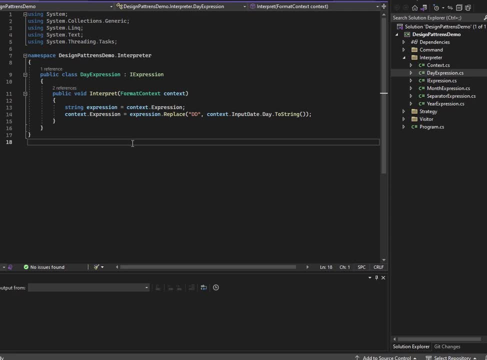 Okay, So, as I already explained, a very simple interpreter which basically takes a date time value, basically a date time constant, and formats it as per my need, which, or as per my, as per the format I'm passing to my client application. 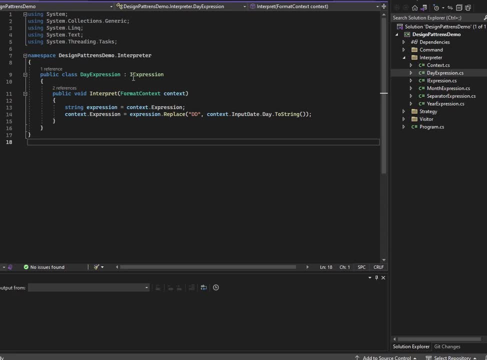 Okay, So a day expression implements I expression. Okay, Receiving the global context object: first thing. first you take that expression, whatever is passed as an input, basically, or whatever desired expression. I wanted Right, The format, the date time format, whatever I'm passing, like DDMMYYYY or YYYY MMDD. 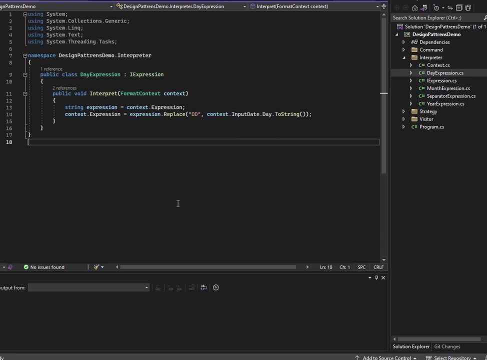 So whatever format I want to achieve. So what I'm going to do is First I will take that expression, put it into this variable, Then I'm going to perform that evaluation. Very simple operation, Okay. On the string variable expression dot, replace the placeholder DD by the context dot: input date: dot: date, dot to string. 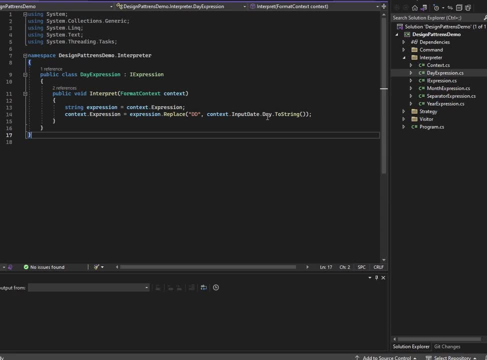 That's okay. Basically, it returns me the day value. Okay, So this DD will be replaced by by day. That's why it's a day expression. Okay. So I would say it's a terminal expression. Okay, It will straight. 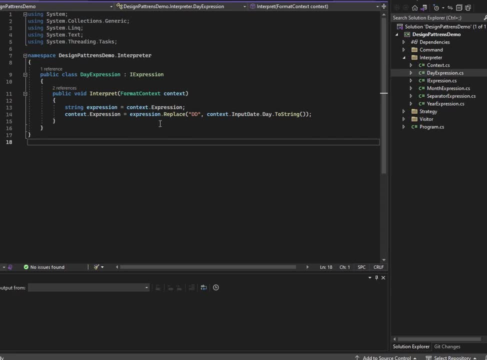 Away, returns a value or assigns a value or basically modifies the value in your expression coming from the context object. Okay, So that's what. So day expression basically takes the DD value, replaces it with the actual day. Okay, For the input date, whatever you have passed, same way month expression, same global context, get the expression value. so that see the reason of passing this context. 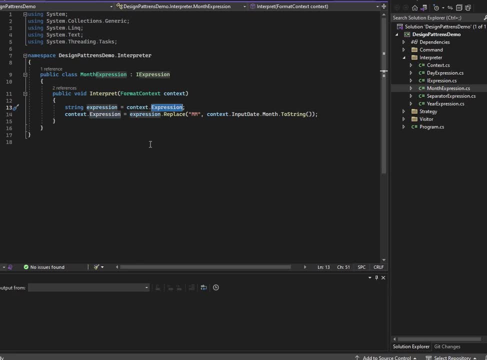 As globally- is that whenever you interpret each and every part of your expression- right, okay, or the pattern basically, or the desired date format you want to achieve- each and every part needs to be interpreted and that will be replaced by the actual value. 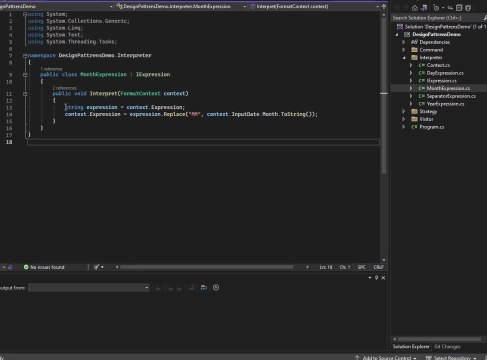 Okay, In real world applications again, the implementation will be very complex if you consider the programming languages or the interpreters which basically parse your SQL Server SQL statements. Okay, So this is a trivial example. So what I'm doing, I'm replacing the month value by the supplied month in my date. 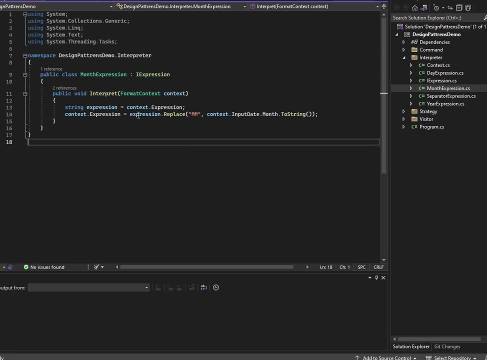 Time input. Okay. So again, see, after performing the operation replacing the month, I'm assigning it to the global context expression itself. Okay, So, based on the input password, the desired format is passed. Okay, Based on that format, this expression value will be getting each. 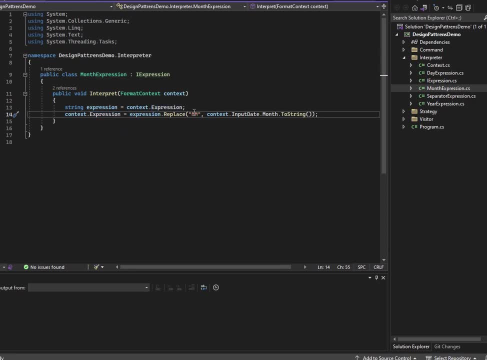 And every uh, place holder value, place holders being replaced by the actual values. okay, guys, so if i go to here, so same thing: get the expression context or expression equal expression dot. replace this four character y, y, y, y by the actual year string. very simple one, okay, and then the separator. 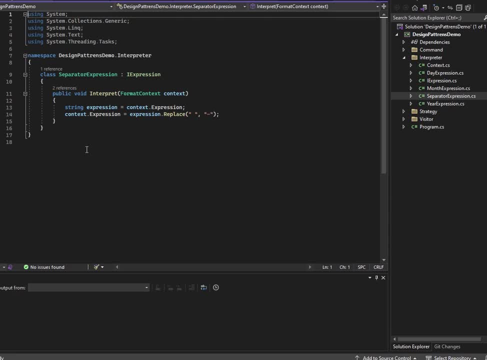 expression okay again, because i'm expecting some formats, which i'm going to show you soon, like dd, slash, mm, slash, y, y y y, rdd, dash, mm, dash, y, y y y, something like that: okay, day, month, year, year, month, day, this kind of combination. so in the given uh expression, if, if the input has the date. 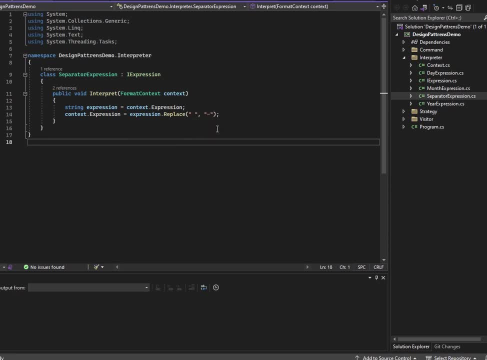 month, year separated by space, then my desired format needs to be replaced by the hyphen value in order to separate those constants. so in my small example i'm making use of dash to separate this month, uh, day and year values basically. so that's the separator expression. 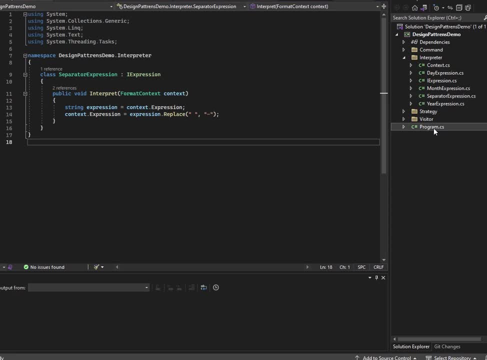 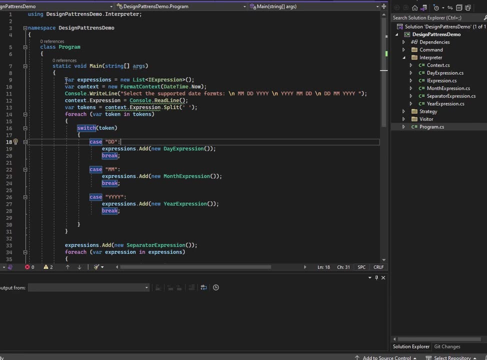 so let's move on to the programcs now. okay, so first of all, i should maintain a tree for expression, but as it is a very trivial example, guys, i'm just maintaining a list over here because my example, or my purpose, is to get a formatted date. okay. 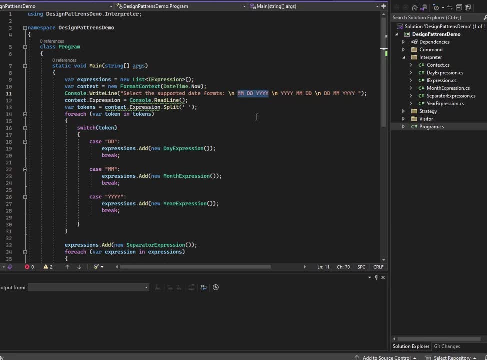 now, in order to format a date, i'm not required to perform any mathematical operations. okay, it doesn't contain any arithmetic operations. so here, uh, composing my expressions into tree doesn't make any sense, so this is a linear operation. so i'm maintaining the expressions list, okay? list of. 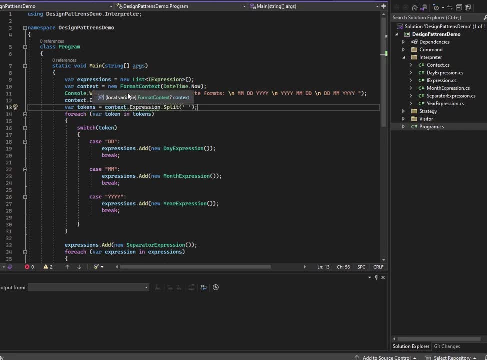 i expression. then i'm initializing the context, the format context, and see this value: date time dot. now i'm passing the current date time value over here. okay, then i'm asking the user: boss, these are the selected date formats which i can format for you. okay? the interpreter is saying yeah, okay, so either you can select, either you can enter this as a input. 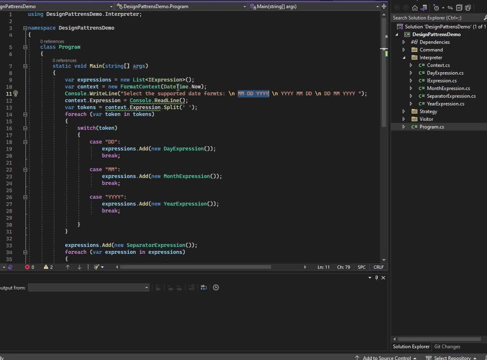 so that it will be formatted with this format for the given date, time, timestamp. okay, uh, either you can give this format or this format, okay, and then you read the expression so the user will enter any one of this. basically, okay, very simple. so i will read that expression and then i'm going to enter. 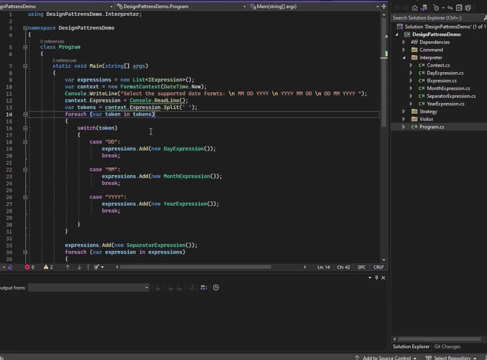 the expression, i will split it by space. okay, then, for each token that is yam, that is month, day, year. what i'm going to do, basically, i'm going to construct the expressions now. okay, so if the token is date, then expressions dot add. for this collection i will add a day expression. okay, if it. 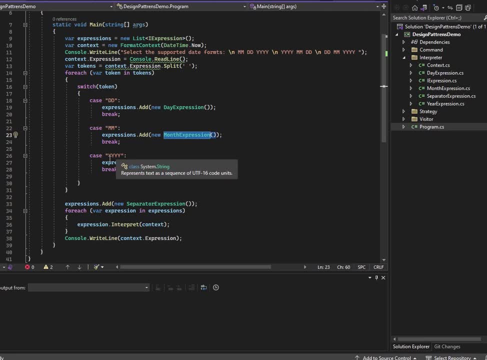 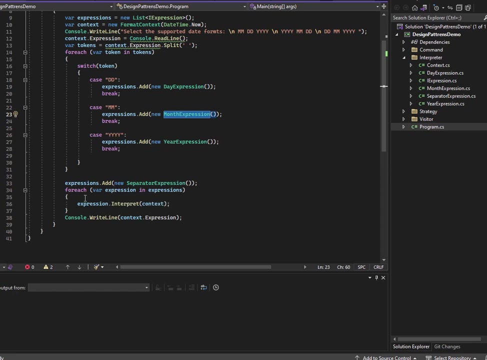 is month expressions, dot. add a month expression. and if it's a year with this placeholder four y's, then it's a year expressions. okay, and then, in order to separate these three values, i'm making use of a separator expression which basically puts a dash. then, once all these things are done, i will run a for each loop, for each expression. simply, i will. 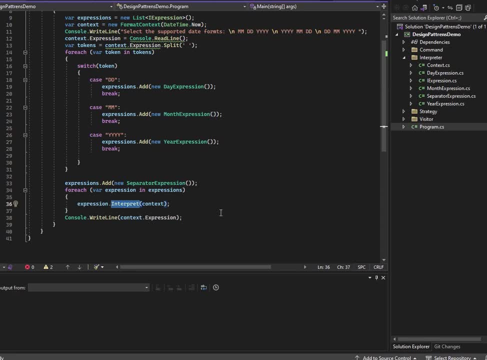 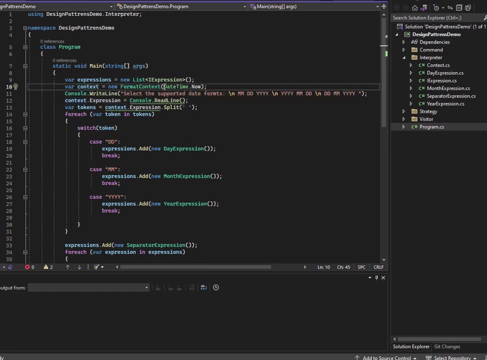 call the method: interpret. that's what the pattern is: interpreter pattern. so expression, dot, interpret. and the most important stuff to uh understand over here is you need to pass the global context which is over here. okay, because your context contains the input value which you want to format, that is, your date, time, and then your expression, the context expression. 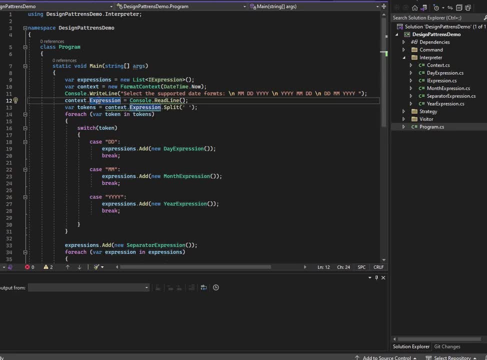 basically the desired format. okay, also contains this expression. basically contains the desired format you have entered. okay. so always remember: the context object contains the input and also it contains the output value also. so this expression, whatever you enter here, only this string literal over here: okay, the placeholder string. basically these placeholders will be. 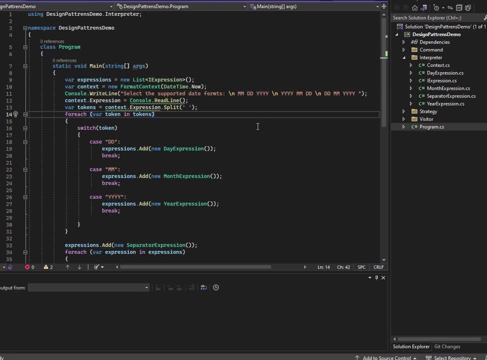 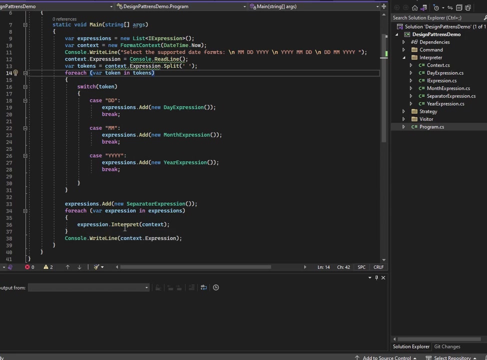 replaced by the actual values. okay, the actual implementations are even complex, very difficult also and very time consuming in order to implement such kind of natural language interpreters. but just for demonstration purpose, i'm making use of this example. okay, so when i call the interpret method, what happens is it will basically go, it will call each and every expressions. 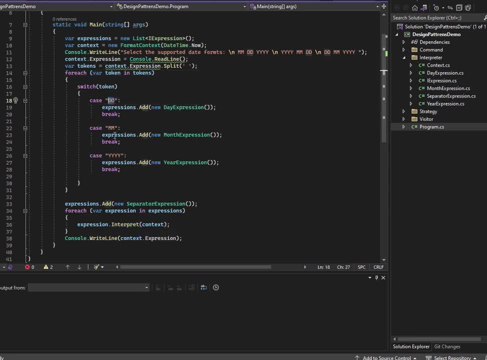 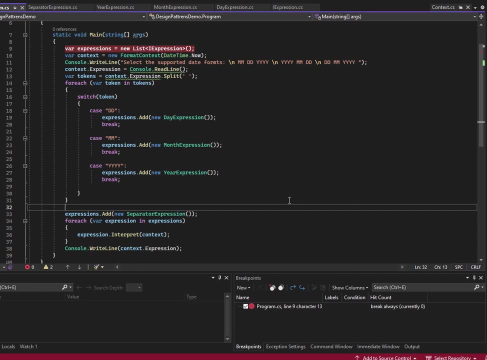 interpret method and it will replace the dd value by the day by day value, month by month and year by year, and also it will take care of putting the dash okay separator. so let's run this program. so let me run the program. so it's running. so initialize the list, or the composite i would say, which contains the expressions: 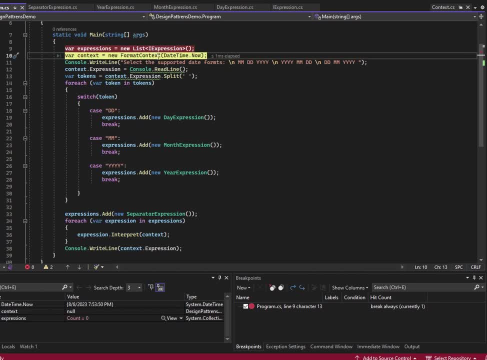 then initialize the context object format- context and pass the time stamp value- the current time stamp value- and then initialize the context object format context and pass the time stamp value. and then initialize the context object format context and pass the time stamp value. okay, then i'm asking user to pick a format. okay, select the supported date formats. 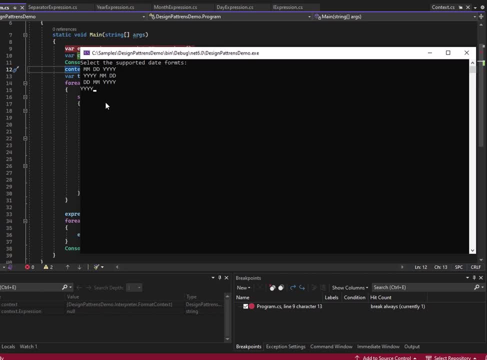 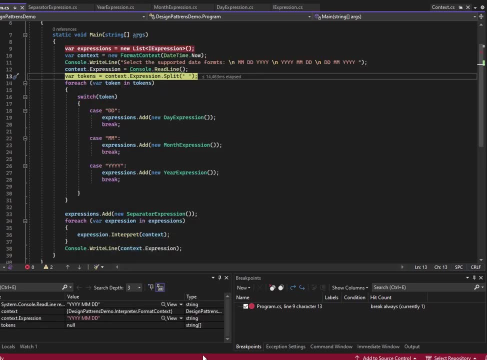 anyone of this. so i will go with year, year, year year, and then i will enter month and then enter day. press enter. okay, the expression has been filled with the required format. okay, or you would say the output also. basically so, so each and every token over here will. be replaced by the actual values. okay, so before we go in to this further process, i will say: take the output and the output and then which is the actual value and which is the actual value set as the usual value set. okay, so, after we have done that, so now we have to line up. 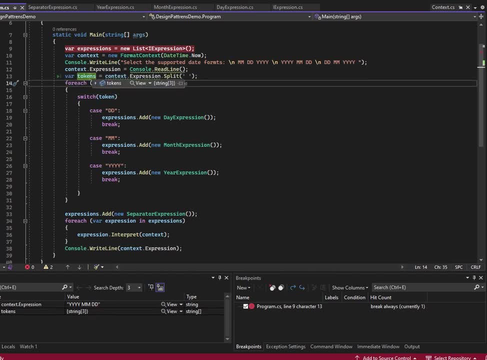 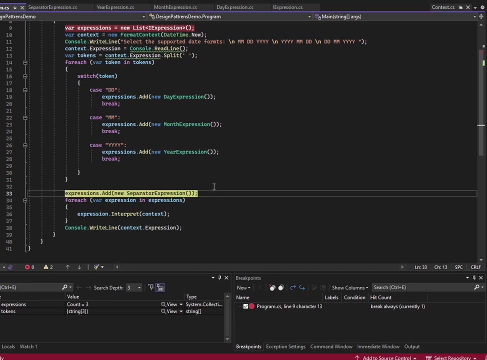 that now first create the expressions. so i split it by space. i have three tokens. okay now, if it is year, put a year expression. if it is month, put a month expression. day, put a day expression, put a separator expression. okay, now we will go to the interpreter. okay, the first expression, which. 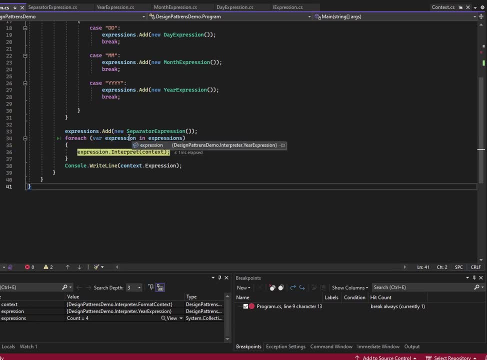 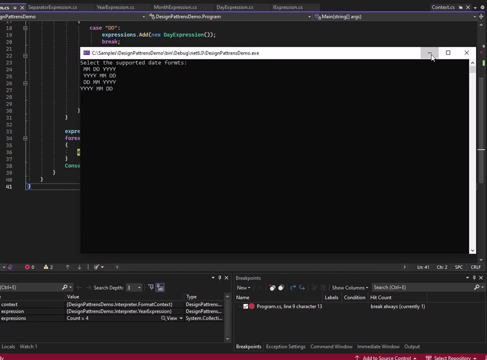 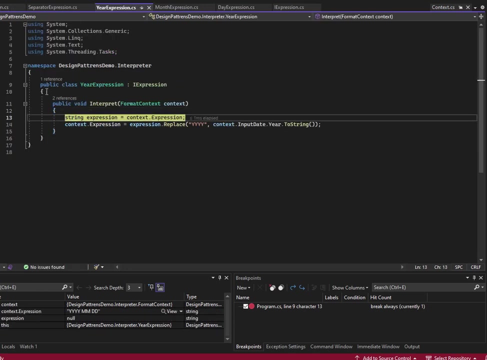 is coming as per the year expression. yeah, as per the format that i have provided over here. so i have gone with this format: year month day. okay, that's why first the month year expression will be evaluated. okay, so if you go inside this, i am inside year expression and my token y y y y. 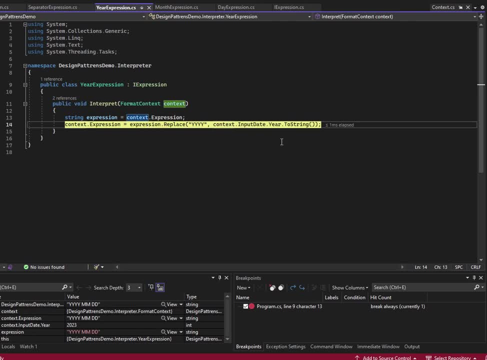 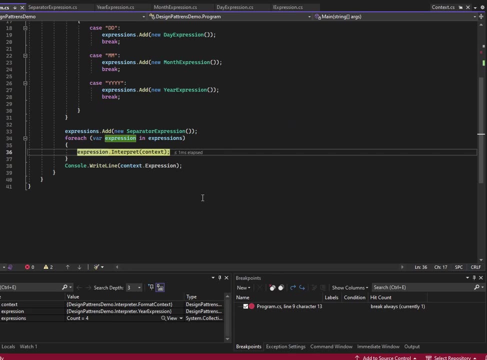 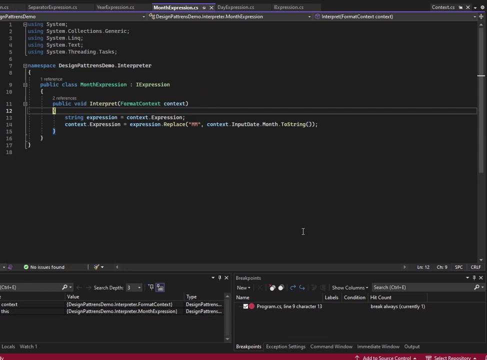 in my expression string okay will be replaced by the actual year value and, if you see, very simple, 2023, mm, dd. okay, now next step, the next token coming over here is now it's a month expression, as per my format. go here, okay, it will take the expression from here, can you see? 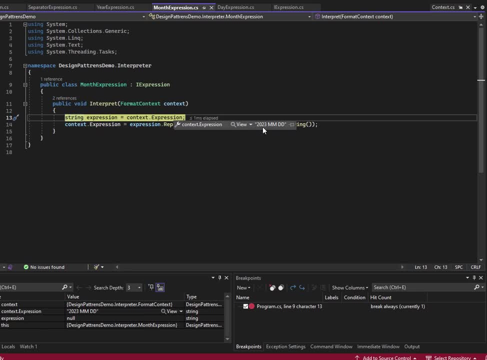 context is global in nature and you can see the changes. year has already. the interpreter meant for the year or the year expression has already interpreted and put its value. that's the year value. now, month will do the job. okay, the month expression will call: yeah, the month. 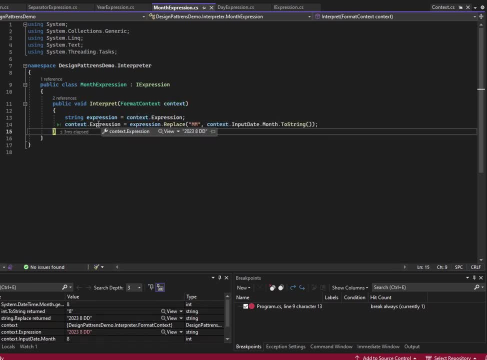 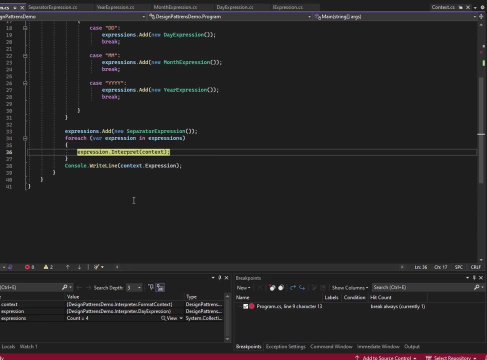 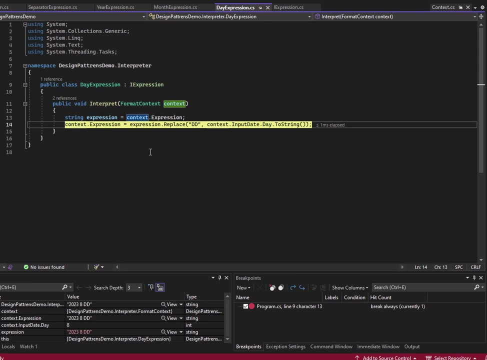 expression will replace this. and if you see, yeah, it replaces it with eight, because month is eight, and then the final one will be the day. fortunately, today's date is also eight. so you see, this, this is your day expression. and if you see, already year and month is updated, only day is remaining. 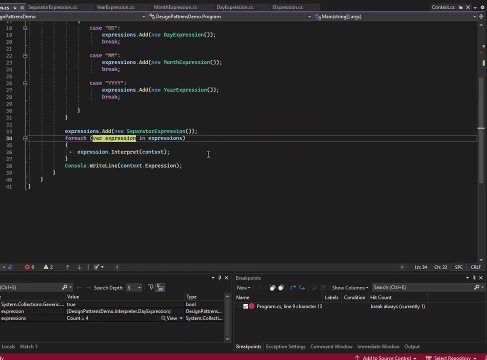 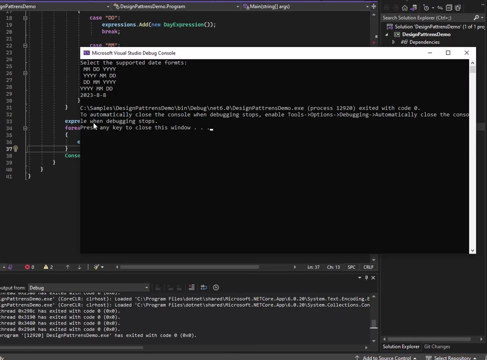 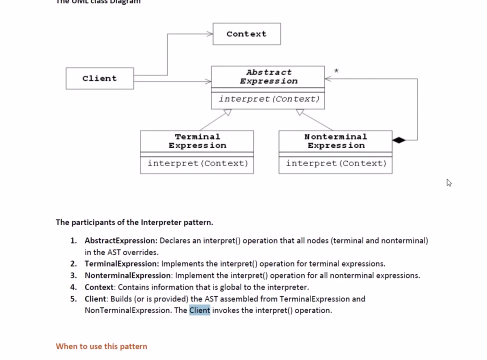 so this will replace d by this. okay, finally, i will print the values. can you see? 2023, month, eight day. okay, it can be further formatted like 0808, but for demonstration purpose, i feel this is sufficient. okay, guys, so this is the interpreter pattern. so let's switch to the pdf. and, yeah, when to use this? 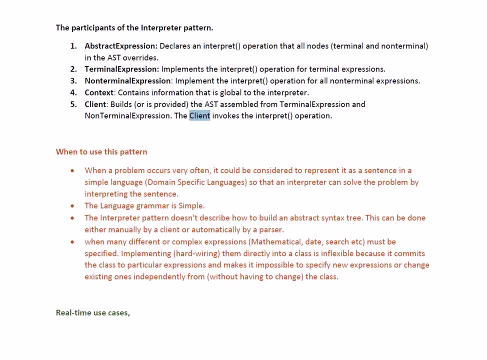 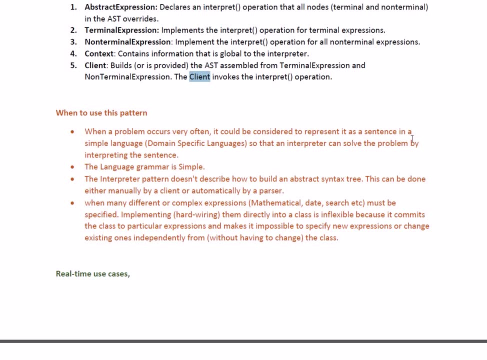 pattern. yeah, when a problem occurs, very often it could be considered to represent it as a sentence in a simple language or domain specific languages, so that an interpreter can solve the problem by interpreting the sentence. take an example of relational databases. when you want to query the records of a table, what you do- you usually do that- select star from table name, update, delete. 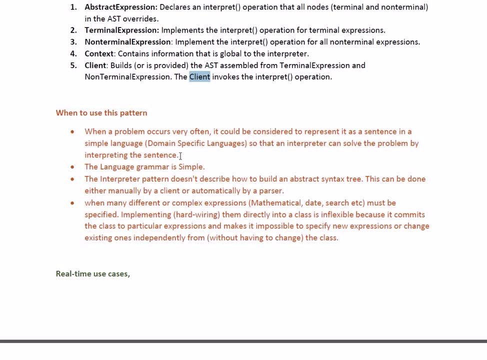 okay, all this kind of frequently occurring operations. that's why they say, when a problem occurs, very often querying the database table, okay, it could be considered to represent it as a sentence in a sentence in a simple language or domain specific languages, so that an interpreter can solve the problem by interpreting the sentence. a natural language based interface so that even a 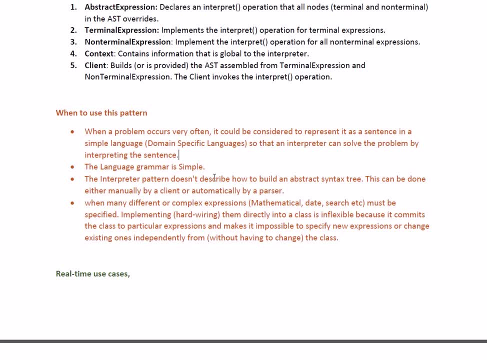 common man also understands and the language grammar is simple. so, as you people would have seen, the language grammar is very simple when, if i take the example of sql, the interpreter pattern doesn't describe how to build an abstract syntax tree. okay, always remember this point, guys. the 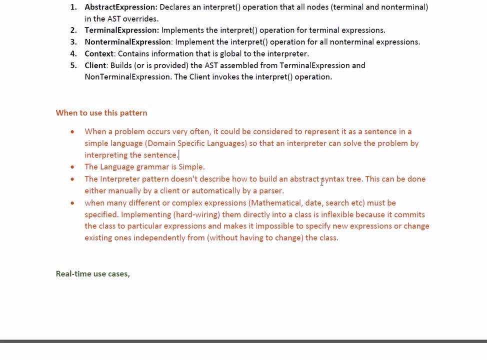 interpreter pattern doesn't describe how to build the ast or abstract syntax tree. okay, this can be done either manually or by a client, or automatically by a parser. it's the responsibility of the parser to build that ast. interpreter only interprets your expressions, that's it. okay, so this is the 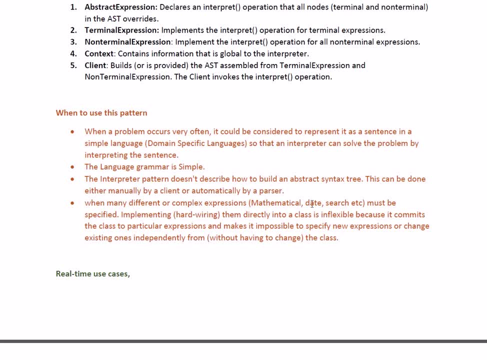 important thing, when many different or complex expressions- mathematical date search etc. must be specified, implementing them or hardwriting them. hardwiring them directly into a class is inflexible. it commits the class to particular expression and makes it impossible to specify new expressions or changes existing ones independently. okay, or change existing ones independently from the class- okay. 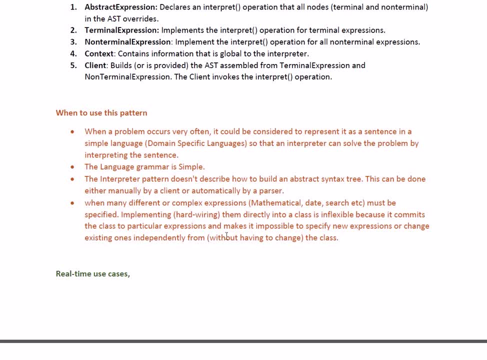 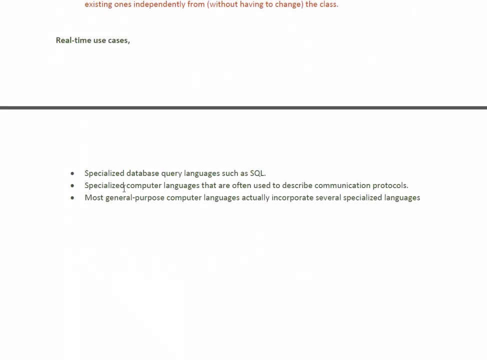 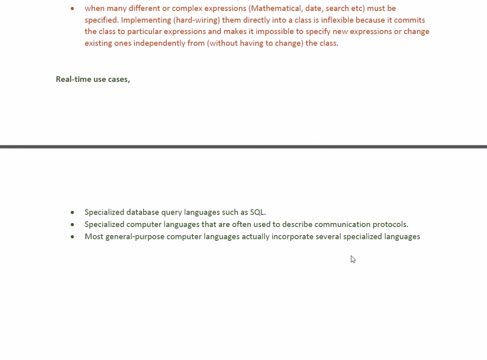 without having to change. so when all these kind of scenario comes into picture, then we need to make use of the interpreter design pattern. real-time usages: specialized database query languages such as sql. specialized computer languages that are often used to describe communication protocols: most general-purpose computer languages actually incorporate several specialized languages. okay, so. 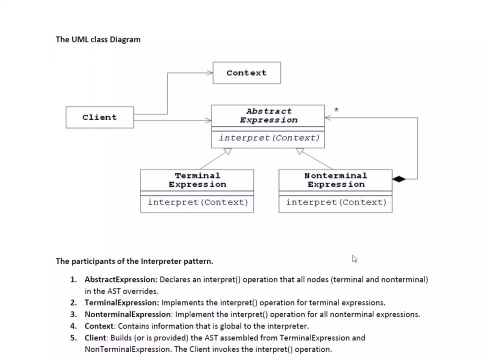 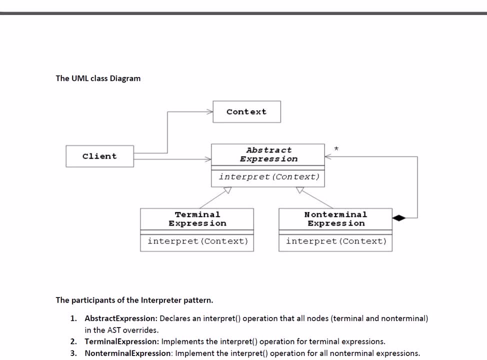 these are some real-time use cases, or i hope you people understood. i think the concept is pretty simple, okay? uh, thank you for listening guys and have a nice day. 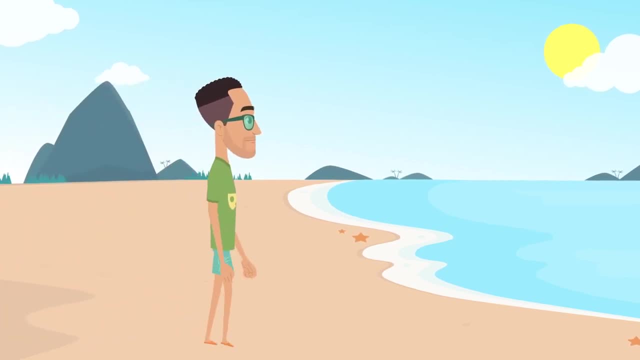 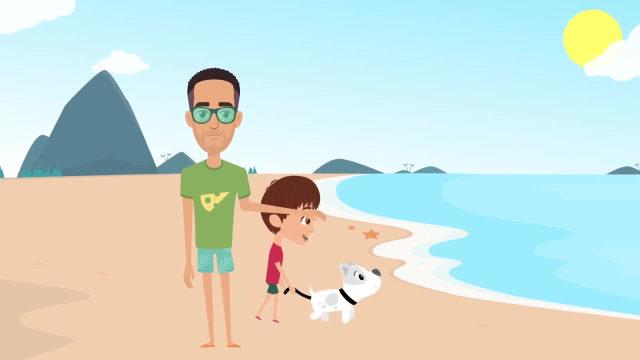 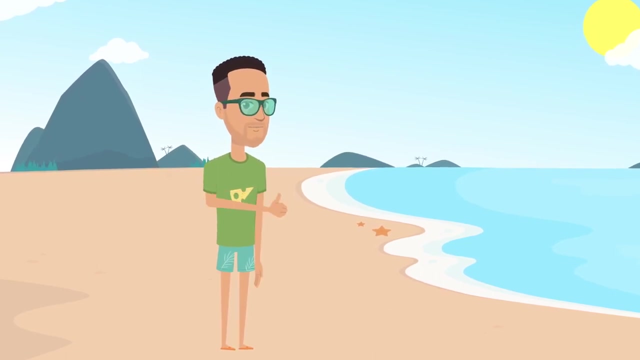 Hello everyone, this is Joe from Team Animaker. In this tutorial, we will see how to create 2D character animations and add voiceovers to them, similar to what you are looking at right now. We bet this is the easiest tutorial that you will ever find. Are you excited? 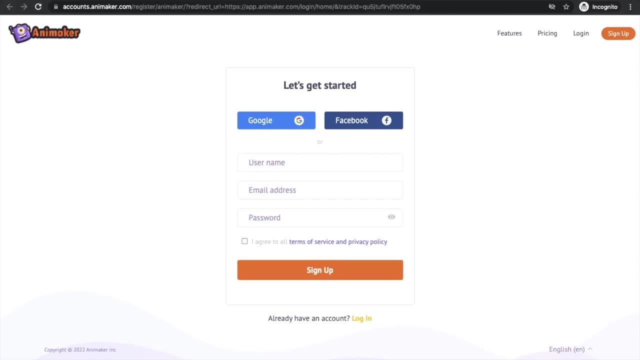 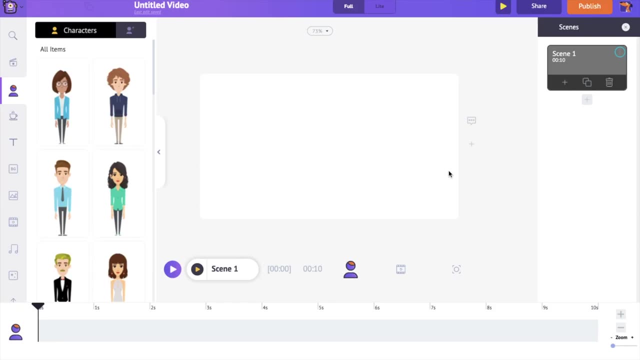 Hop on, let's get started. Visit animakercom and sign up for a new account. On the dashboard, select the following options to create a new video project. This is the interface of the animaker application. In the center is the workspace On the right.